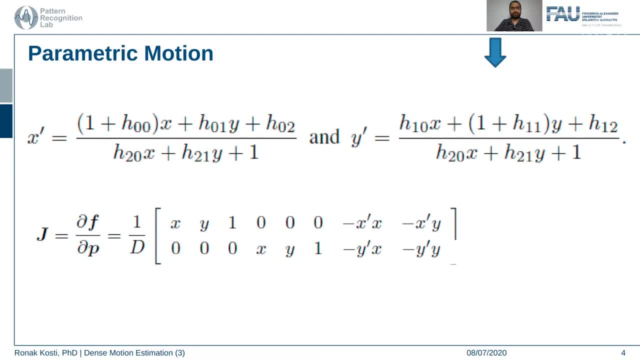 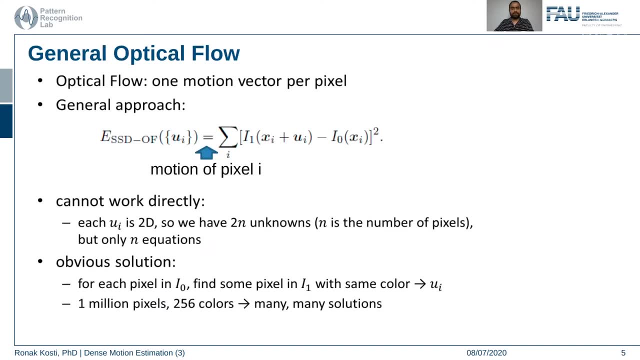 and how many different methods can be used for calculating, estimate or estimating optical flow, Using the generic motion flow or the generic motion estimation of your, between your frames in the video or between two images, So the general, the most general form of optical flow can be represented. 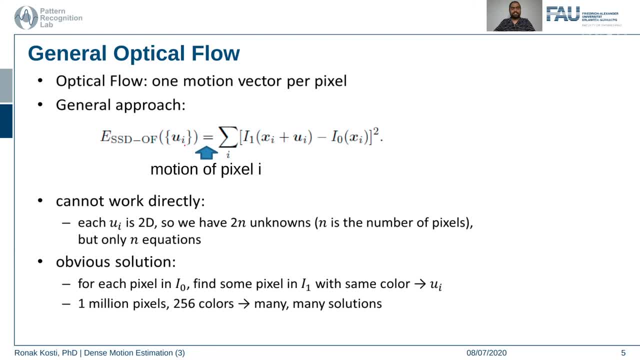 by this equation, where Ui represents each and every pixel in your given image I0.. And so, using this error metric, you can find the motion for, or the optical flow for, each and every picture pixel. This is very dense, and for every pixel you will have a motion vector. However, it's inefficient to 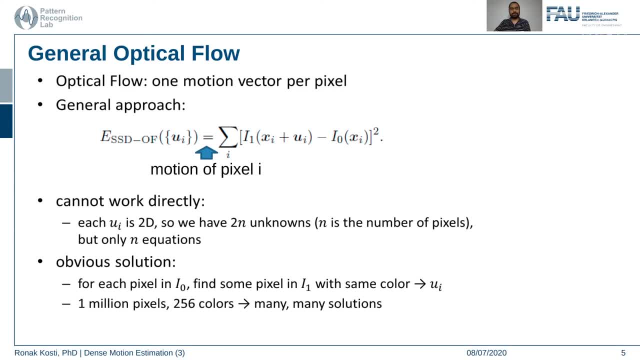 compute. It's a highly complex problem and it has a large number of unknowns and we have not enough information available. And it's not always the case that we need this every pixel level information And the obvious solution. we already know that for each pixel in I0 we find some. 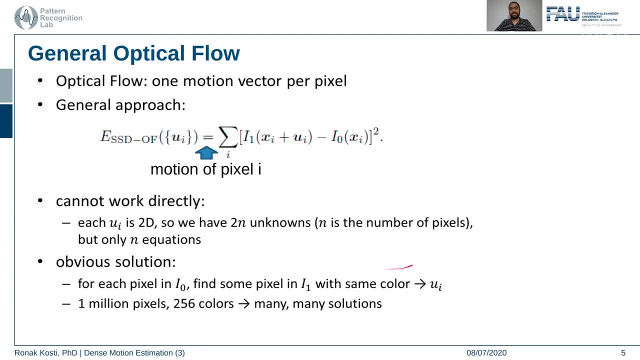 random some pixel in I1 with the same color, for example. So for every pixel you will have. let's say, if you are using an RGB color space with a range of values of 0 to 255, then you can have 256 color for every pixel. And so let's say you have a pixel value of 120 and you just have to look for that. 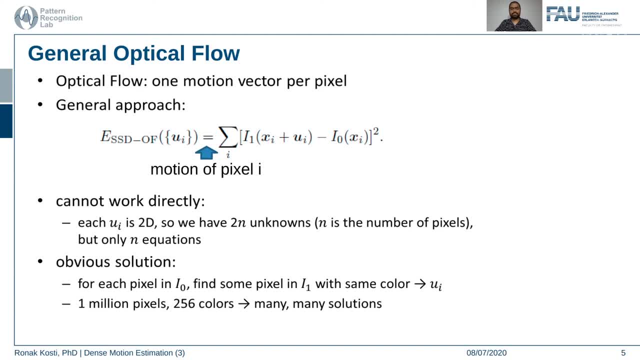 pixel value in your next frame to match these two pixels, So you can estimate the flow between them. But let's say, if you have 1 million pixels in your input image, then there will be in addition with 256 color. there could be many, many solutions And it's 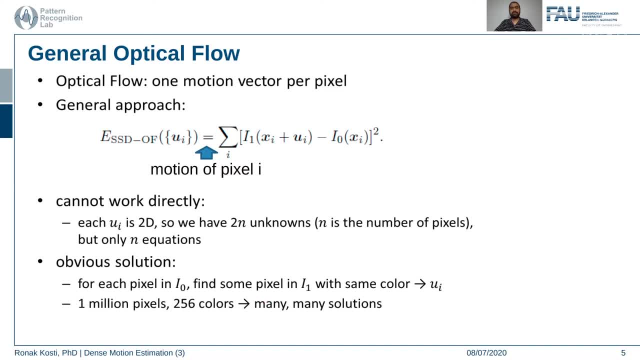 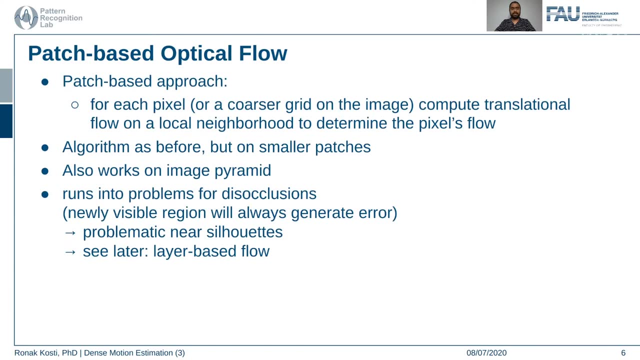 not necessary that every pixel will have a unique solution. because there are only 256 colors, It is highly likely that for every pixel value you have thousands of matches. So this obvious solution will be better. And think in terms of patches. So how do we do patch based optical flow? So instead of 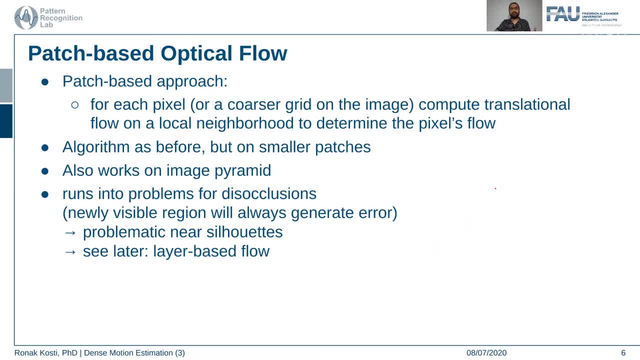 looking in the neighbor in the whole image for a particular pixel value. We look at patches as well. So you have to define some patches in advance and you have to find these patches in the next image and compute the optical flow between them. So instead in patch based approach, basically, instead of 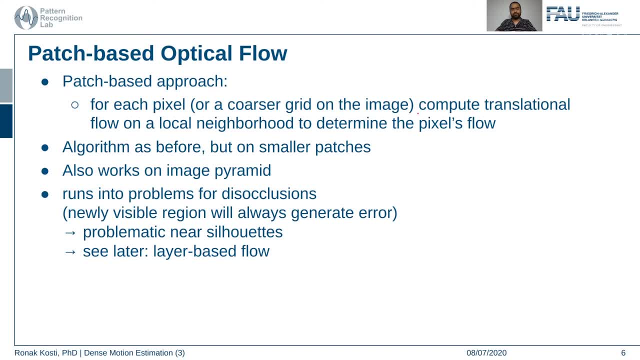 pixel. you have a local neighborhood for which you determine the optical flow or its pixel, for its determine the neighborhood to find the optical flow. what it means is that you fix your neighborhood in your reference image and you look for that kind of that neighborhood in your target image and 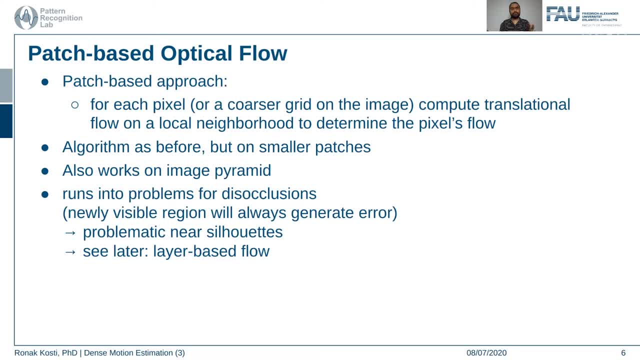 when you find this matches, then you compute the optical flow for your given pixel value. okay, you can use this patch based approach using the same algorithms as we have discussed before. you can also use image pyramids as a feature extractor or a feature scalar to use patches. so if you reduce, then image. 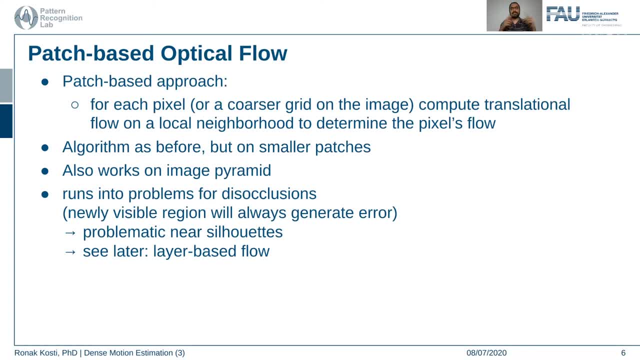 scale to the coarsest image scale. there it's easier to form patches and then you find optical flow over that using this patch based approach and then compute it for your whole neighborhood of the pixel and then slowly scale up and then you refine your optical flow vector as we have discussed in the previous. 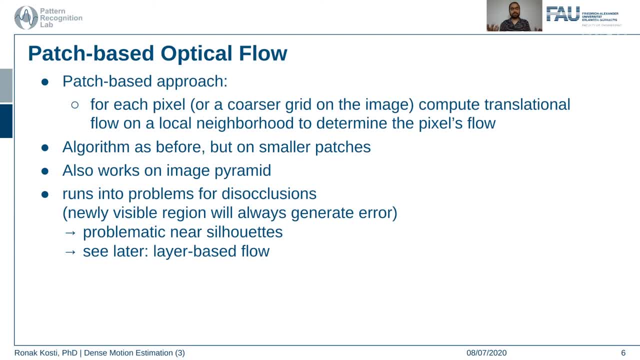 part and in an iterative fashion, and so on and so forth, and you will find, for your original image scale, the final optical flow value for each and every pixel. however, this problem is not the most efficient because, let's say, if your image is too high or if the frame difference between the two frames, for 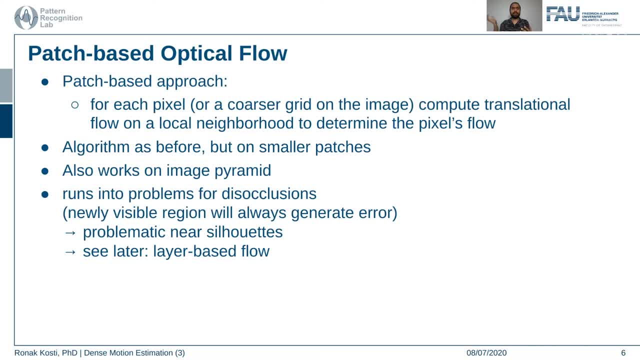 which you are calculating, the optical flow is too high, maybe a new object appears, for example. a very good scenario is monitoring traffic, right, if you are traffic, if you are, if you, if you are trying to take two images separated by a few seconds, there are a lot of different new cars or automobiles coming into your 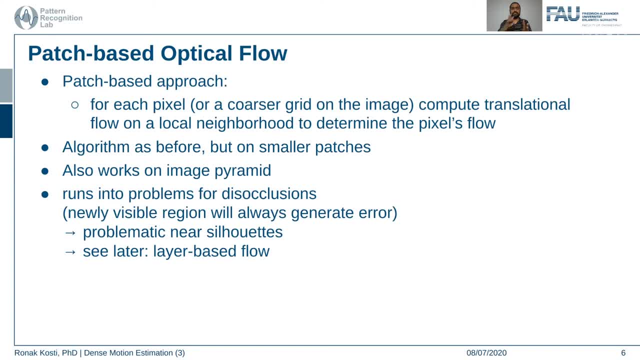 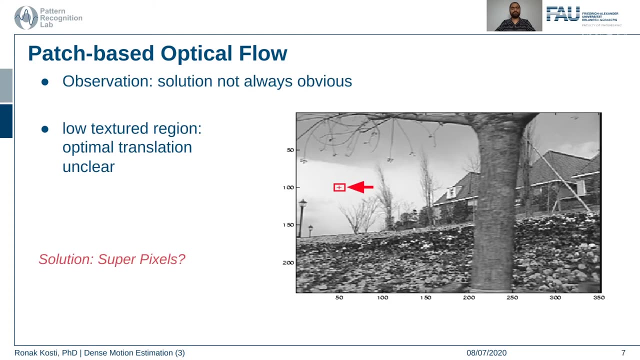 image frame and a lot of objects which were there in your previous frame have left. so, because of these occlusions, because of this addition and removal of new objects, because of this motion, it's not always easy to go with the patch based approach. so, for patch based approach, let's recap in a way what we 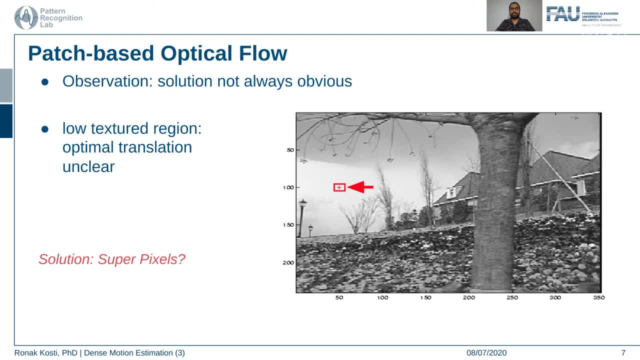 did before for feature matching. our feature extraction is to find this reference patches right. you have to find this feature matching. there is a number of features which are matching in this two different images and then you find: define this local neighborhood using this features and then you find the optical flow based on that. so the 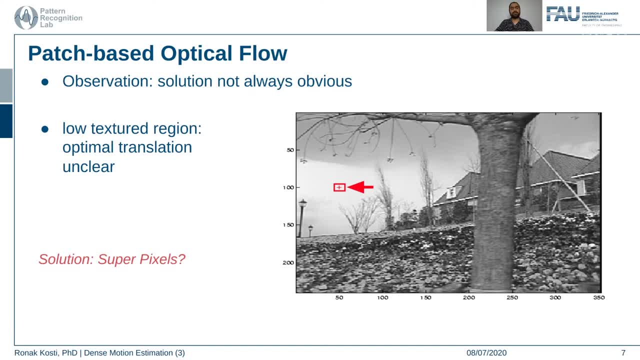 natural question comes to the mind is: what features are the best? right- and we have seen this before in our feature matching, feature extraction lecture series- is: if you, if you take a low textured neighborhood and there are not, there is not much features here, So to define a neighborhood of these features is quite difficult. 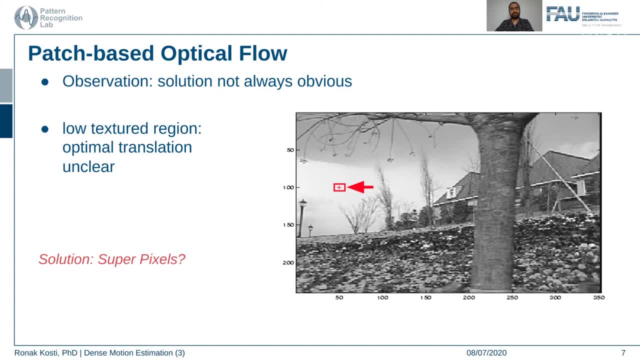 And it's not easy to find a translation from this region into a feature. So we need more distinctive or discriminative features such that it is easy to match the feature from one image to another image. So essentially here you are also trying to solve a correspondence problem by finding 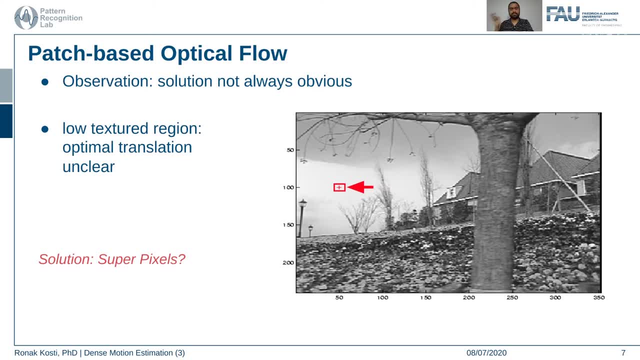 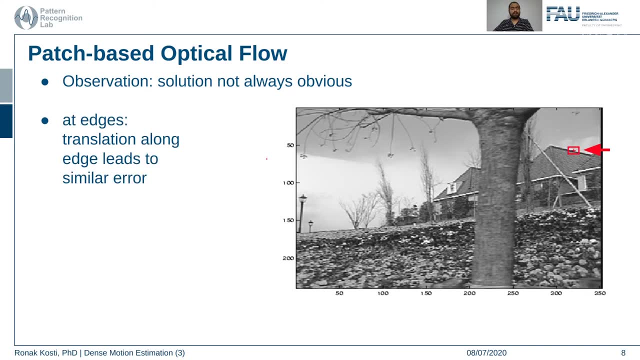 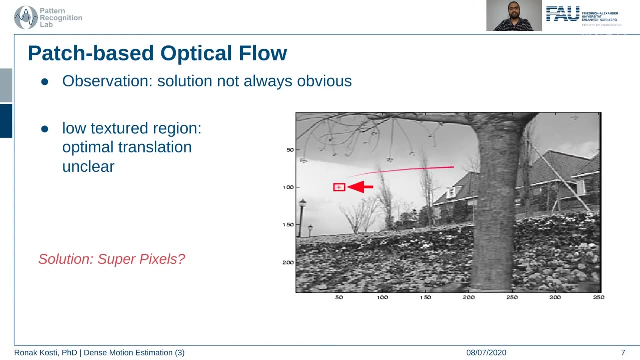 a matching pixel values or matching feature values and then you find optical flow for each of your pixel for that neighborhood. In the edges also, it's a bit better than using any low texture regions, because in edges if you go in this direction then the features do not change as much, whereas if you go in. 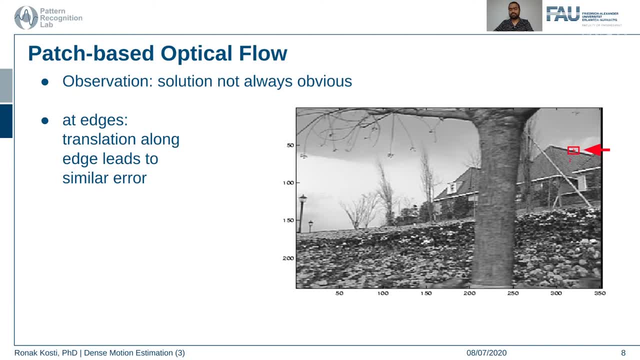 the horizontal direction, sorry, the perpendicular direction to the edges, then the features will change dramatically. So this direction can be used for patches, for finding these patches, but they are not. they might. you might end up in similar errors, because if you find similar edges somewhere else in the image then you are doing, then your correspondence is incorrect and ultimately, 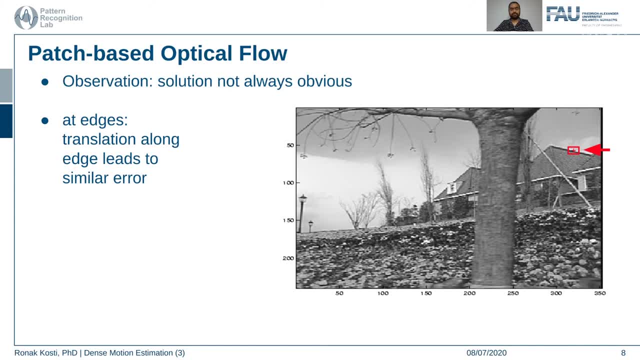 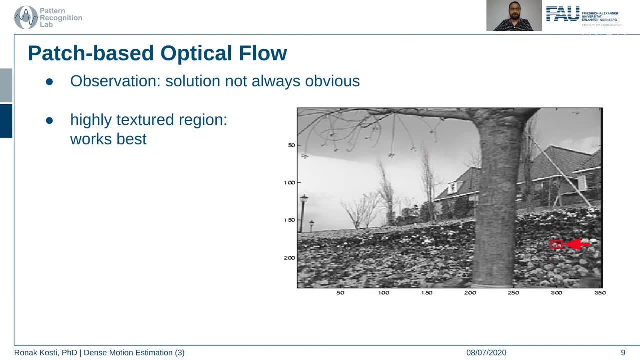 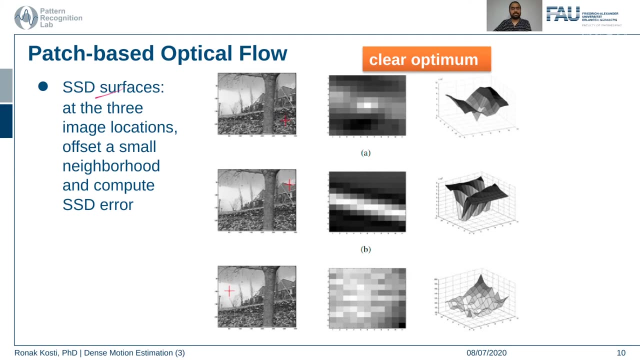 your calculation or estimation of optical flow will also be incorrect. So this is a very important point, Thank you. So we go basically towards more higher textured regions which work the best, which we have already seen for corner detection as well. So essentially what it is is: you find this sum of squared different surfaces at three. 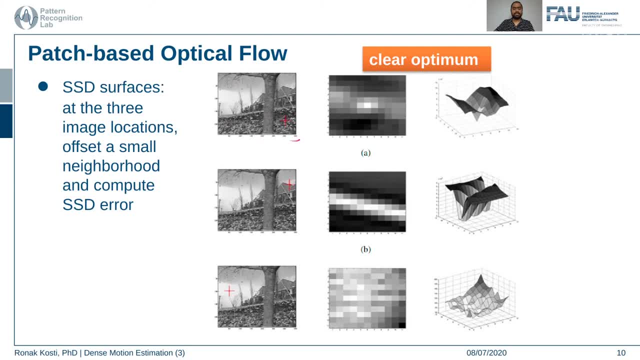 different image locations when we have seen here in the high textured, in the edges and near the low textured image and the neighborhood will give you a very nice local optima here. There is a clear optima when you have, when you are finding a surface or patches for a 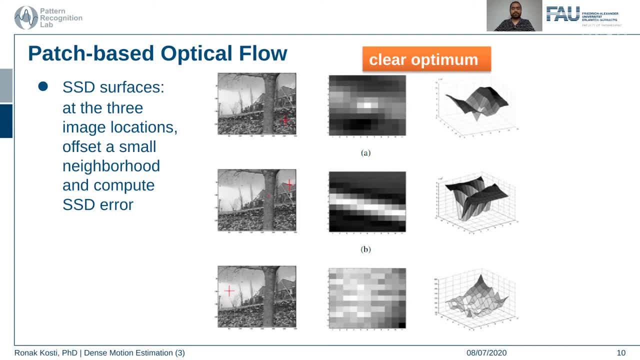 neighborhood which has a high variability around it, whereas for edges it is. there is sort of a valley. So if you go in this direction, it is unclear and there are multiple solutions possible. Similarly, if you have or if you are looking to in a low textured regions, you will get. 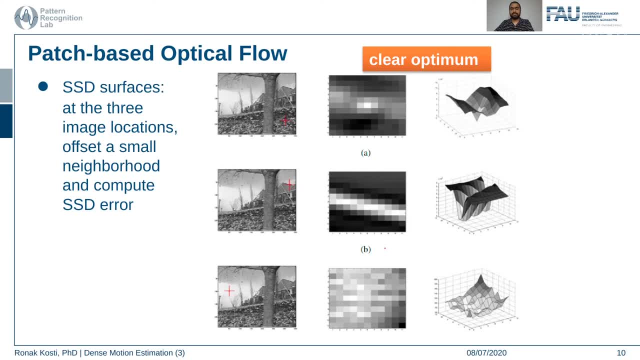 a lot of local minimas Or local optima And therefore it's not a clear answer or a clear solution for your optical flow problem. So we have seen that again, in case of patch based approaches, the best way to go is to find regions which have high textures or high variability or high feature distinctiveness. 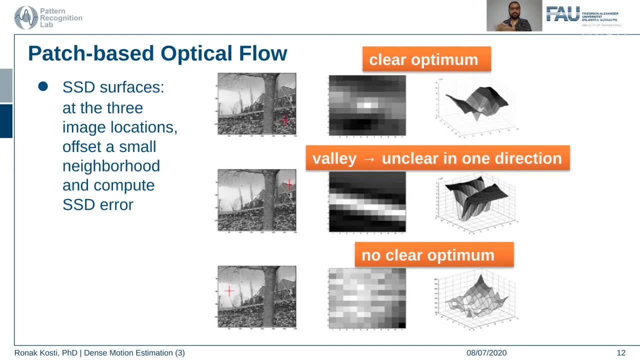 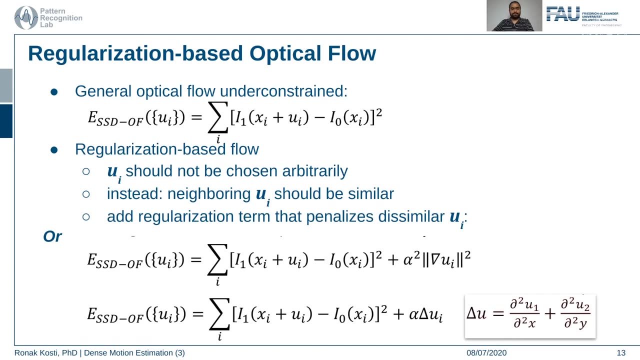 And so it depends on a lot of factors, on what you are doing. in this image, for example, it's clear to see that this region will have Very distinctive features, and that should be the direction to go. OK, so how do we the general optical flow without any constraints, without any additional information? 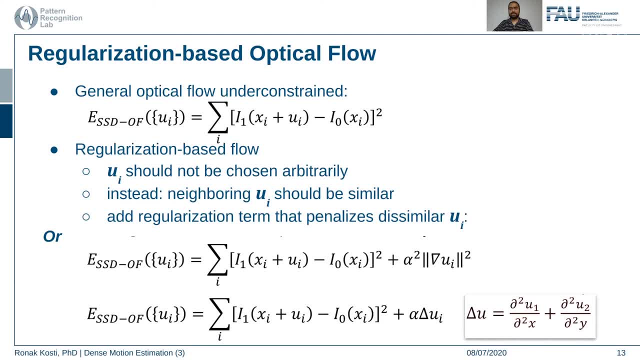 prior knowledge or additional parameterization. it can be represented as sum of squared differences of optical flow for each and every pixel. In this form this equation is quite naive and this shows the basic definition of solving optical flow is minimizing this error metric. But we can include some regularization ideas or some regularization constraint, because 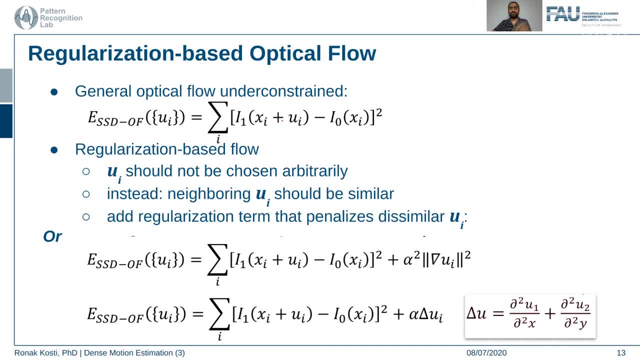 we know some things in advance and we can use that to influence the error metric To reach an optima faster. So what can be done is we know that UI. we should not choose some arbitrary value or an arbitrary pixel. we should choose instead UI such that it has similar neighborhoods. 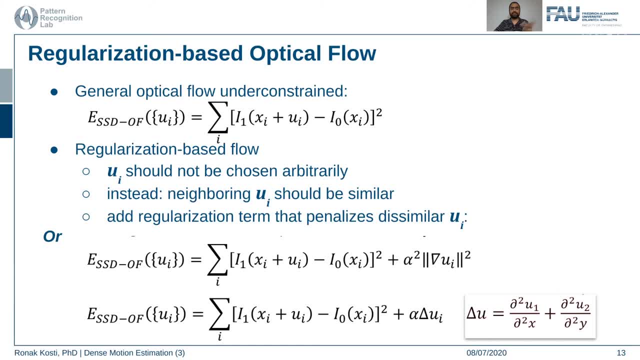 and similar optical flow for that neighborhood. So if you have such a neighborhood, then you can add a regularization term That it's neighbor in the neighborhood. all the optical flow vectors will have similar values and therefore you can penalize the error metric using this information. 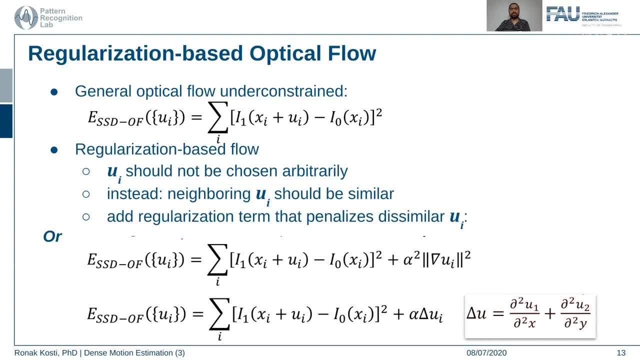 So this is what it is called regularization. So let's say, if you have fixed pixel value or a pixel location in your reference image and you have defined a neighborhood of that pixel, and then you're looking for the same neighborhood in the target image Or in the next frame and you want to compute the error metric here, 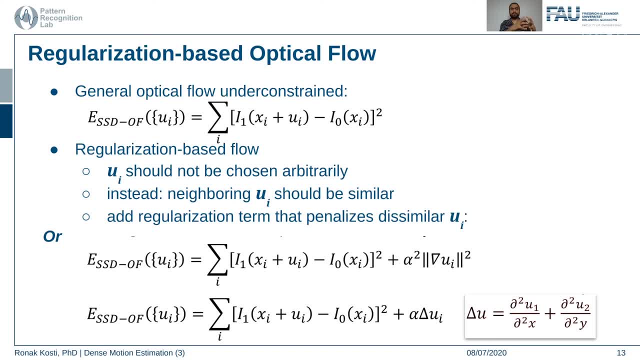 Now, given this assumption that the neighborhood of this pixel has similar values of optical flow, the changes of optical flow will be minimum. So we add a regularization term called the gradient or the delta- sorry, the gradient of UI. So we include a gradient. instead of a gradient, we can include a delta of U, which is represented: 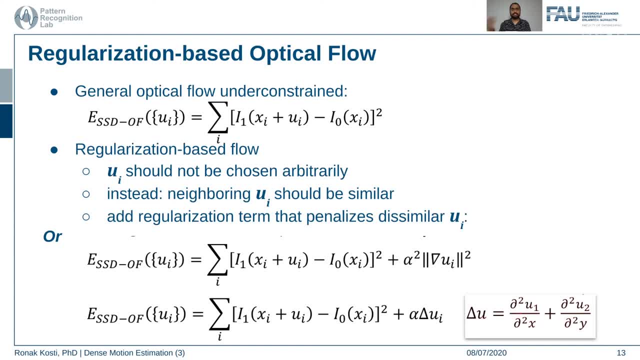 or is just a partial derivatives in X and Y direction. And if you take a partial derivatives in X and Y direction in the neighborhood of UI, it is going to be minimum because it does not change as much as ui, and so this regularization constraint will bring us to the solution a bit faster. this is just one example of regularization. 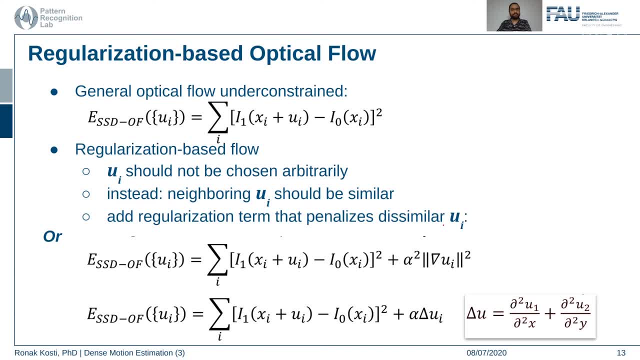 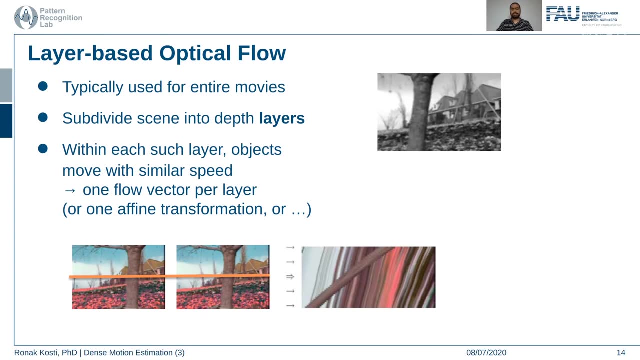 term that penalizes dissimilar uis. however, and that could be depending on the problem, you can find different regularization terms. another way of finding optical flow is layer based. so let's say you have a video and this technique is more popular with animation, generating animations and movie making. so you have set of you have a video which has a feature length. 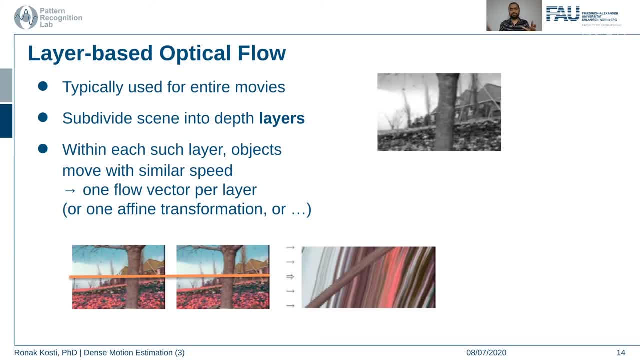 and there are multiple frames which change over time, or they shift or they move. An example is given here on the top right corner. So the method approached here is that each layer is assumed to have a constant optical flow and so the image is divided into different layers, which separates each part of the image. 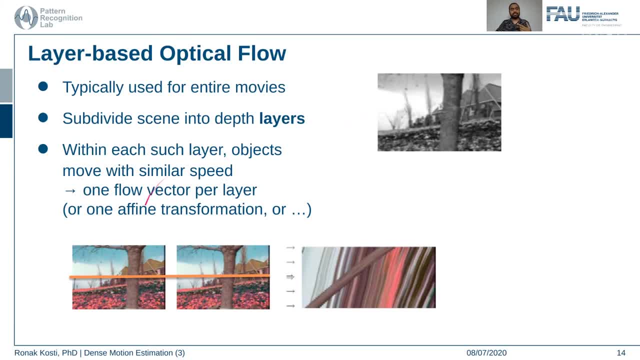 based on its optical flow vector. So what we do here, for example, so it will have one flow vector per layer, more or less what I said. So, to just give an example, what is done here is, let's say, these are the two different frames here, As you can see that the tree, 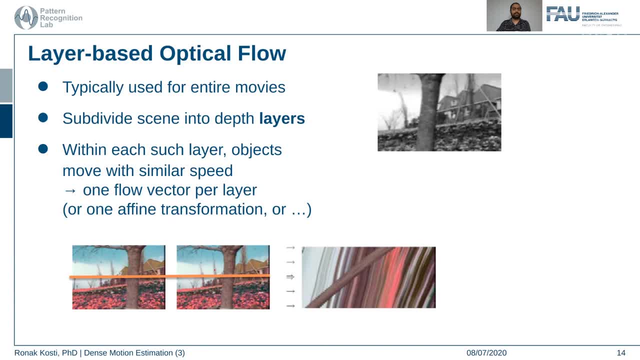 has moved from the left frame in the left hand direction, in the right hand frame, and you draw this line or you take the features along these line in both the frames, then in all the frames in the particular video, and you plot them or you stack them horizontally in this direction. okay, so when you do that, you see that the 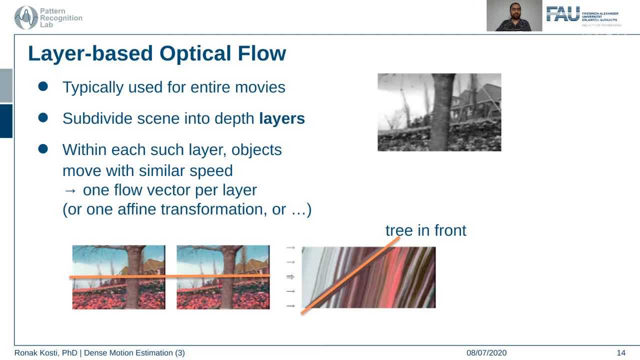 tree has a high the the tree in the front, the features on this tree moves quite fast, and it's apparent from this motion as well that an objects nearer to the camera center moves faster than the objects away from the camera center, which also we have discussed in previous parts. so here it is clear that 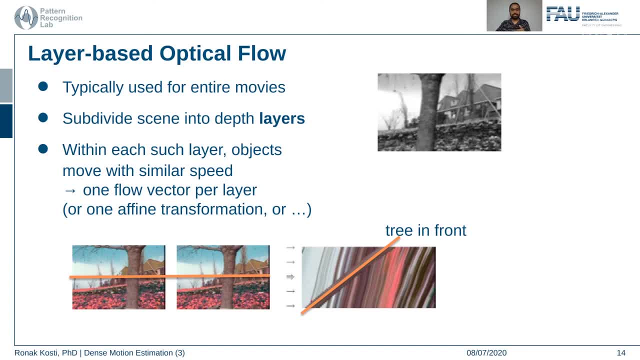 this tree trunk is visible which has a higher speed of movement along the frames than the other parts of the video. so, for example, the tree in the back, it moves slower, or, yeah, it moves slower than the tree in the front and using this information, you can assign specific optical flow. 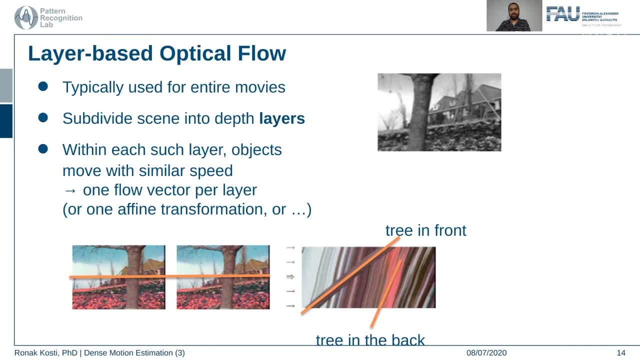 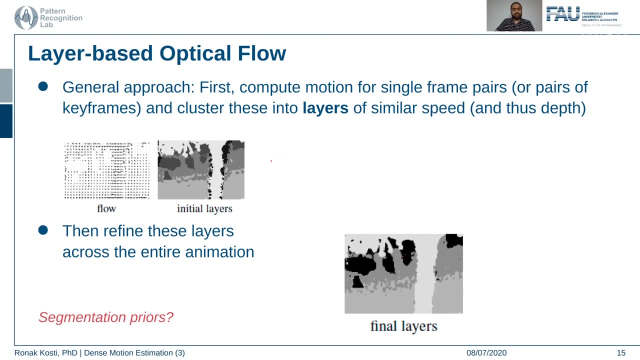 values or optical flow vector per image layer, and then compute the overall optical flow and hence you will get final motion motion estimation for your image. so the general approach for layer based optical flow is: you take pairs of, you start with pairs of frames first, you generate the flow vector or the, which is the most. 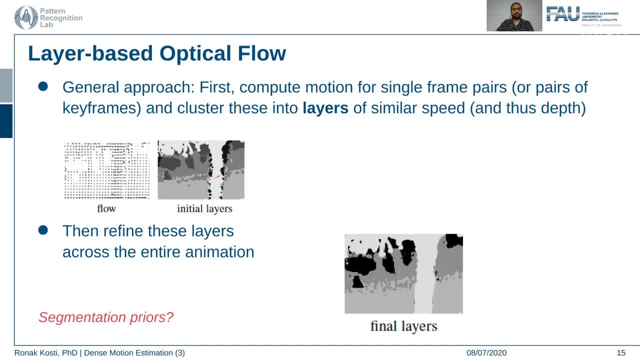 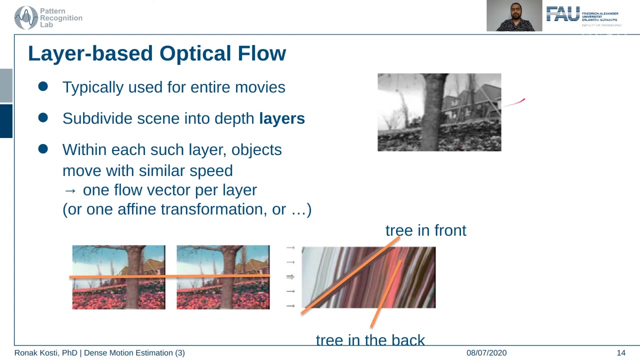 coarsest or the most roughest estimate of the initial layers, and then you refine this layer across the whole animation to finally achieve a nice-looking optical flow vector. when, when you look at this diagram here, it looks like you are looking at some segmentations as well. so based on this moment, it's easy to segment different. 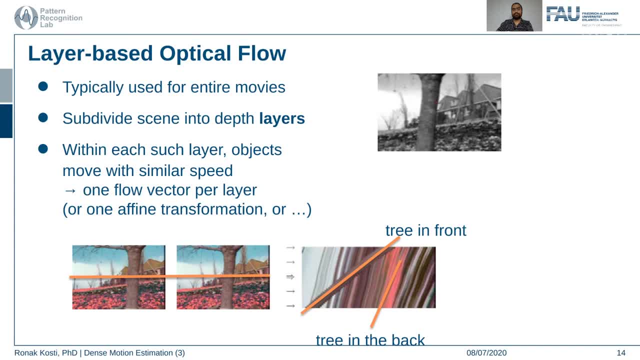 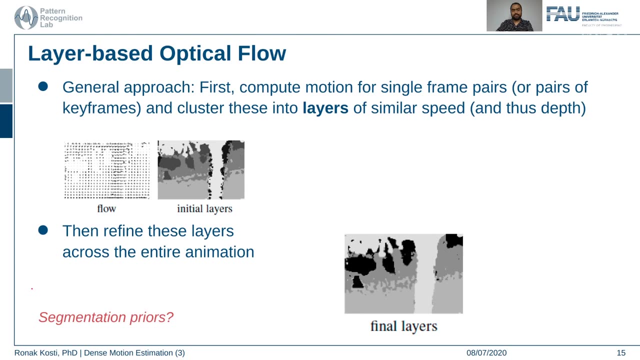 parts of the image and because if one object, for example this tree, it's a one single object and if you track this tree across frame, you're essentially also indirectly solving segmentation problem. so the question here is: can we use this flow information, optical flow information for as a segmentation prior? 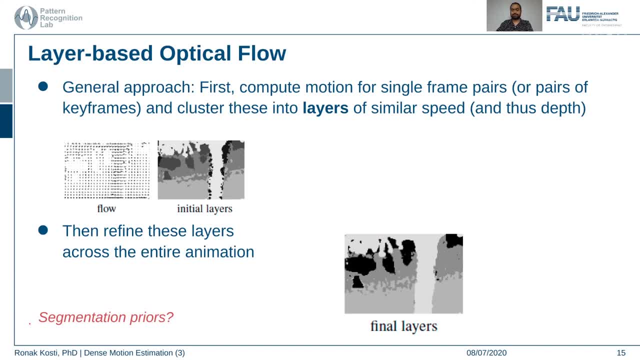 for solving segmentation task. there's something to think about. it's not part of the lecture, but it looks quite nice that how an optical flow generated on a for a video can also essentially be used for segmenting the different objects in the video. that was the most basic way of solving optical flow through layer based. 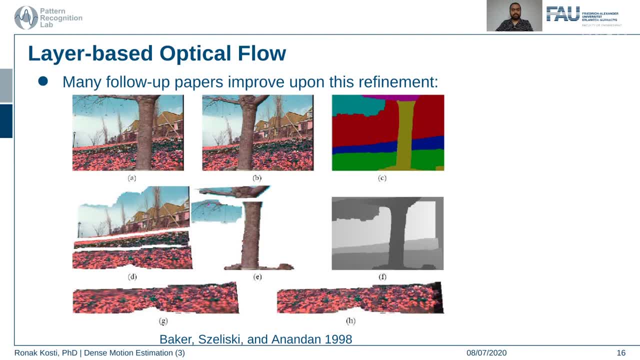 approaches. many follow-up papers have come, and I mean these days convolutional neural networks and deep learning has solved or created more, better, state-of-the-art solutions to this problem. I for a for a good start of this kind of papers I would recommend you to go and look at. 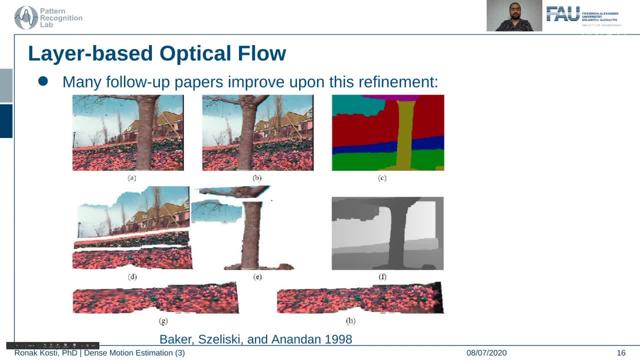 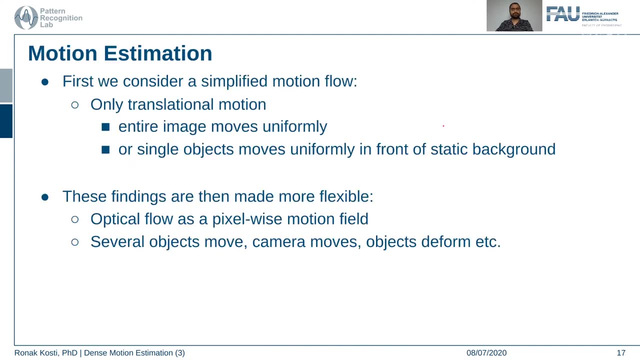 this paper. here they have given a good analysis of a lot of different state-of-the-art and they have also produced nice-looking optical flows which also look similar to segmentation. okay, so motion estimation. so first we consider a simple motion flow, only translation motion. we then which, whenever the entire image moves uniformly in one direction, or a single.